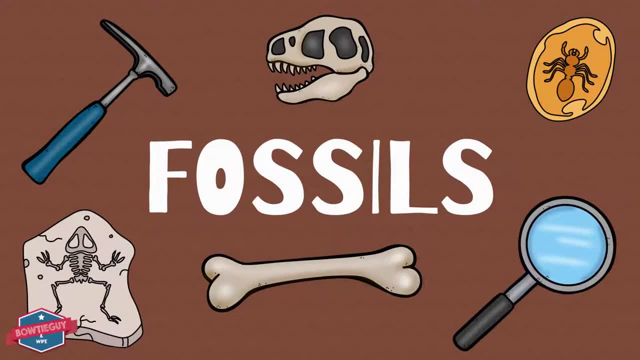 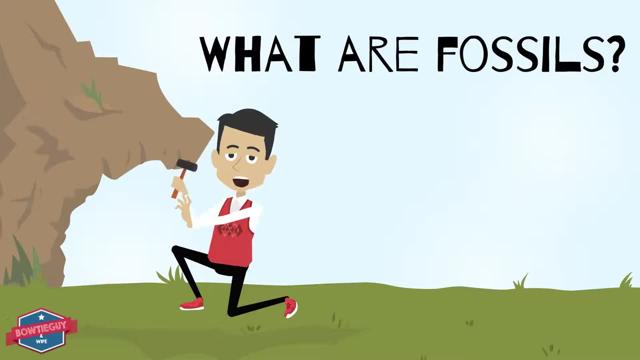 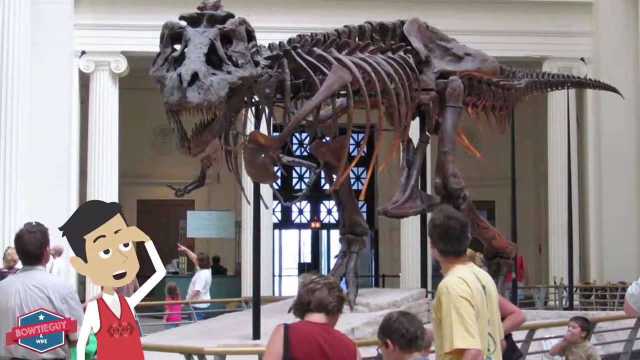 On topic for today's episode. we are going to talk about fossils. Fossils have been found on every continent, on the United States, even in Antarctica. What are fossils? How do we know the dinosaurs even existed? Well, we know from evidence, Evidence from fossils. 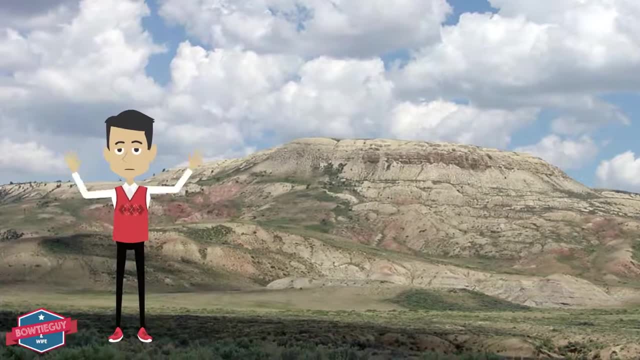 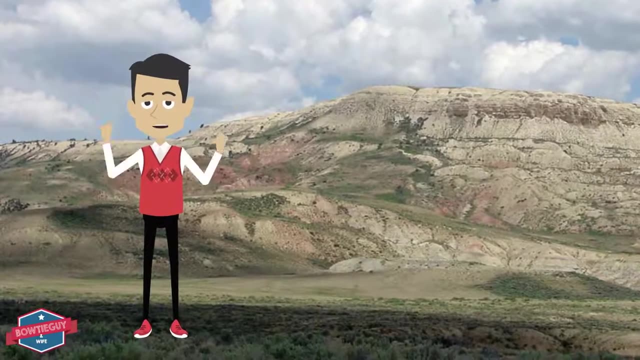 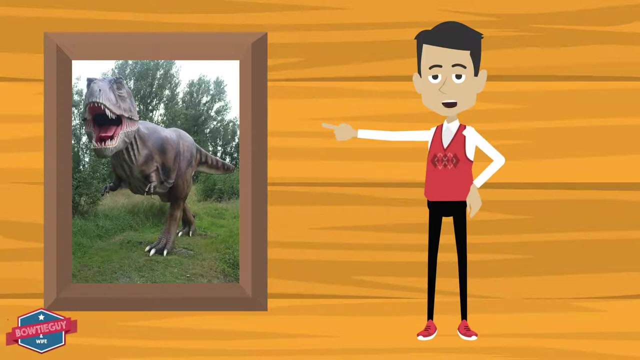 Dinosaur bones can be found scattered over a large area, and scientists must then figure out how they are fit together. Dinosaur skeletons are very much like bird and reptile skeletons, which helps to work out which bone goes where The Tyrannosaurus rex lived 65 to 85 million years ago. 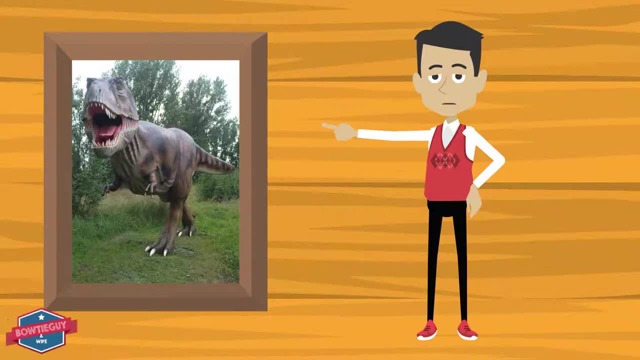 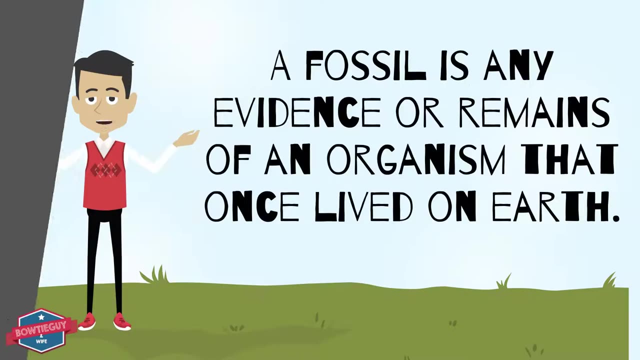 It is now extinct, gone forever from the Earth, But its story, including how it lived and what it ate, remains forever in the fossils that it left behind. A fossil is any evidence or remains of an organism that once lived on Earth. 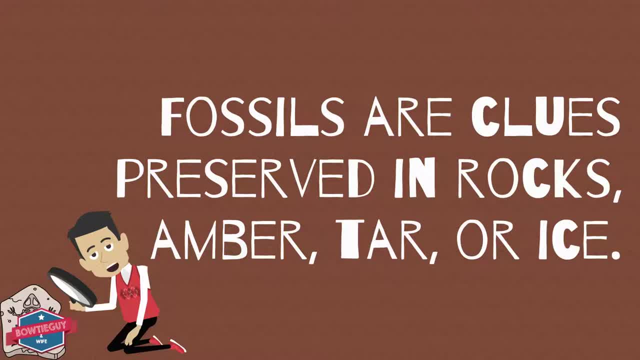 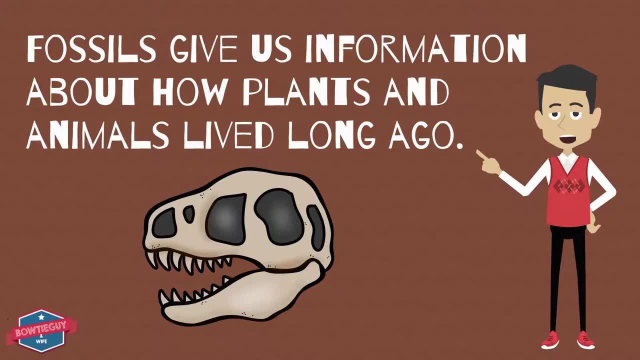 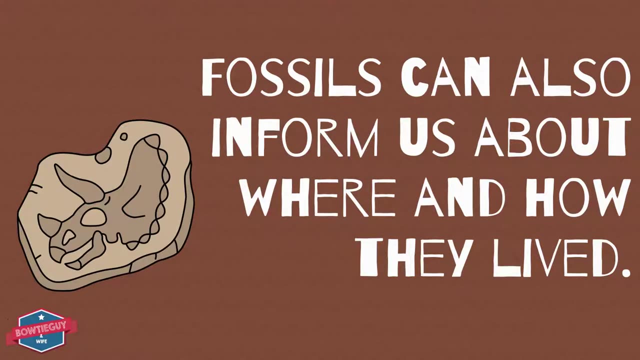 Fossils are clues that are found in rocks, amber tar or ice. Fossils are storytellers in a sense, in that they give us information about how plants and animals lived long, long ago. Fossils can also tell us about where and how the plants and animals lived. 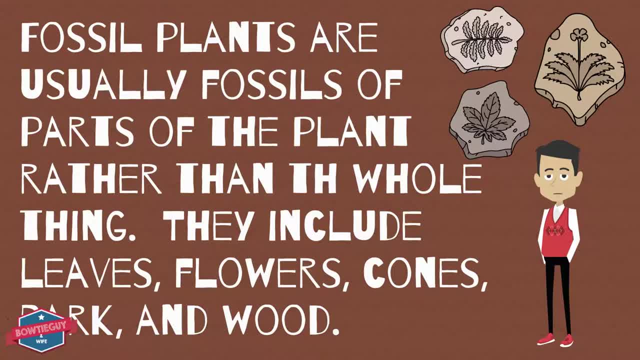 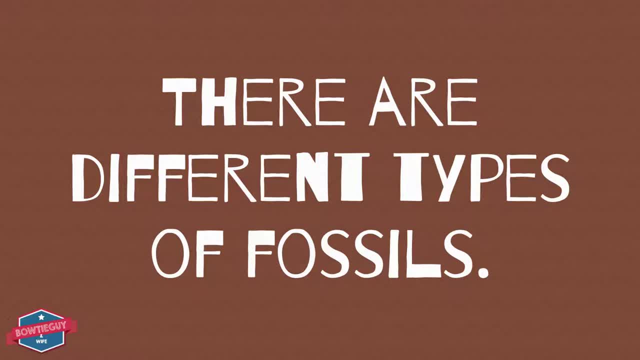 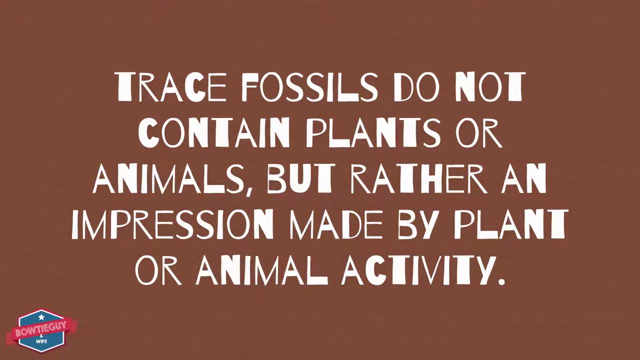 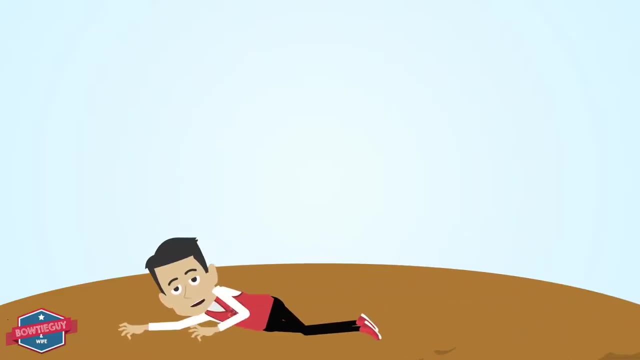 Fossils are found within sedimentary rock layers. There are many different types of fossils. First, let's talk about trace fossils. Trace fossils do not contain plants or animals, but rather an impression made by plant or animal activity. As I track across this mud, I'm leaving tracks. 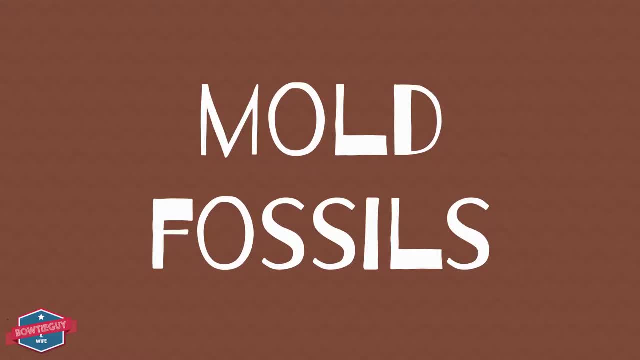 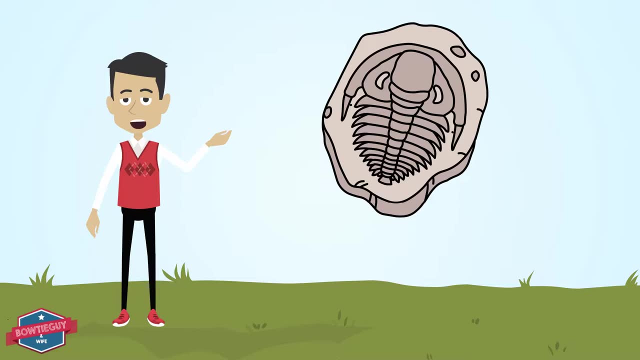 This is an example of a trace fossil. Next, let's talk about mold fossils. A mold fossil is a hollow space in the exact shape of the organism. Here you can see an example of a mold fossil. Next, let's talk about cast fossils. 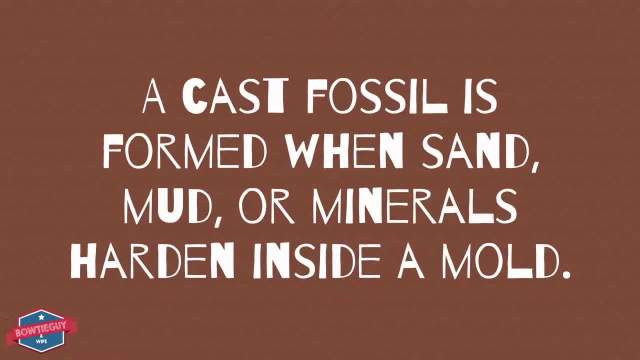 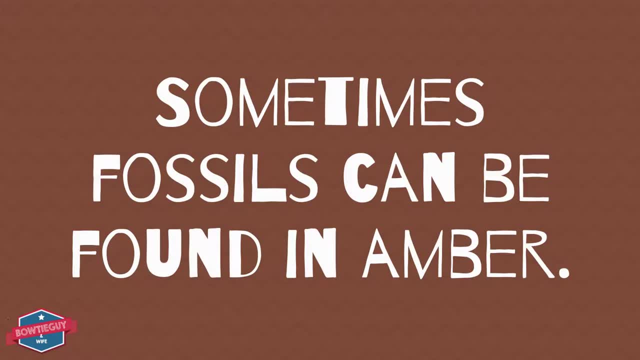 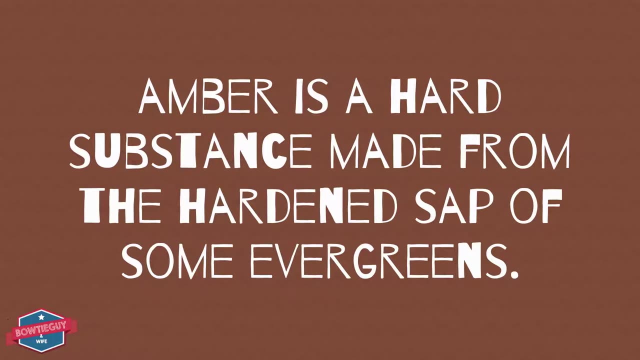 A cast fossil is formed when sand, mud or minerals harden inside a mold. Here is an example of a cast fossil. Sometimes fossils can be found in amber. What is amber? Amber is a hard substance made from the hardened sap of some evergreen trees.